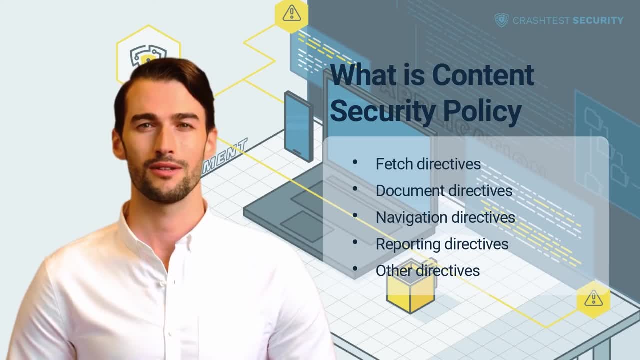 web workers: Connect SRC specifies the URL to be loaded using scripts. Default: SRC: the fallback directive for all fetch directives. This policy directive defines the default source list for other fetch directives. Object: SRC defines allowed sources for applet embed and object elements. Style SRC provides a 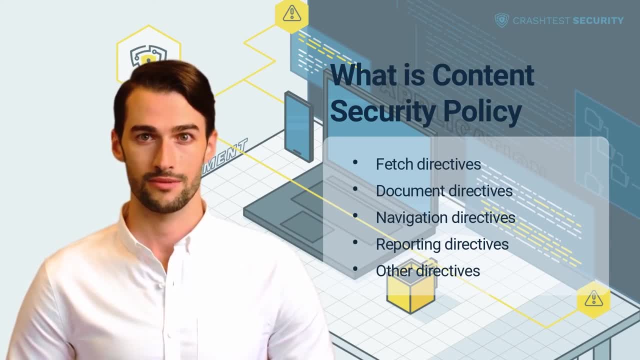 list of valid sources for cascading style sheets: Document directives. Document directives help control the properties of the working environment or document where a policy will be effective. These include: Sandbox: Provides a sandbox for a specified resource similar to inline script elements. Base jury: Specifies the URLs allowed in the document's base element. 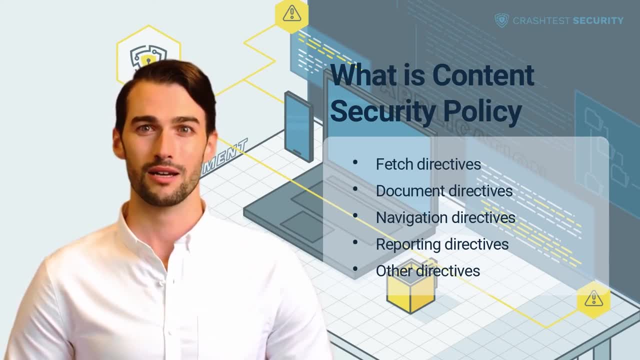 Navigation directives. These directives govern the locations of a form submission or where the document initiates any navigations. They include: Form action: Specifies the URLs that act as targets for the submission of form elements. Frame ancestors: Restricts the parents to be embedded on the web page using the frame. 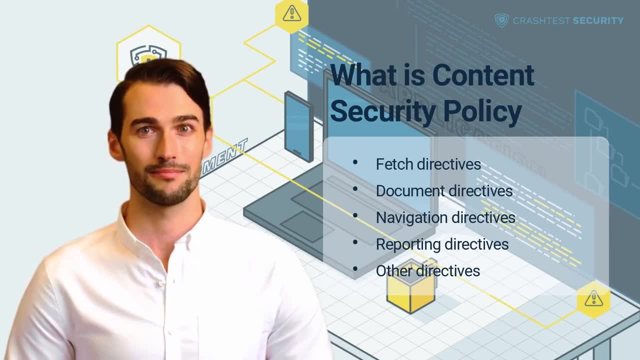 object: eframe, applet and embed elements Reporting directives. These directives govern how CSP violations are documented and reported. They include: Report to Initiates a security policy violation event Report. jury- a policy directive instructing the client environment to report any attempt to violate CSP specifications. Other directives include: Require SRI for Enforces. 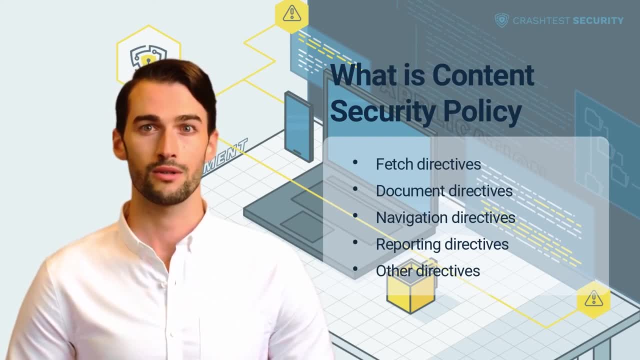 the use of subresource integrity for the style attribute and page script sources. Trusted types Used to specify a list of accepted non-spoofable typed values, Thus mitigating DOM-based XSS attacks, Require trusted types for This policy. directive enforces the trusted types policy on scripts that act as syncs for DOM-based XSS. 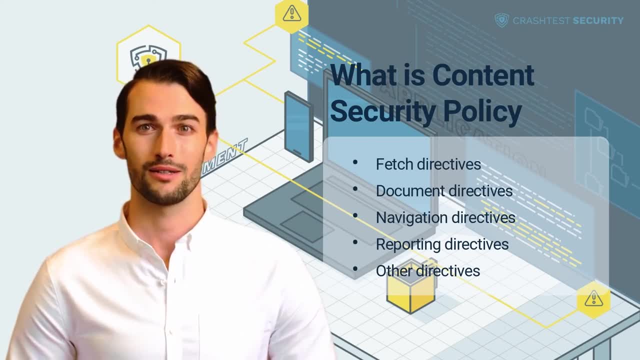 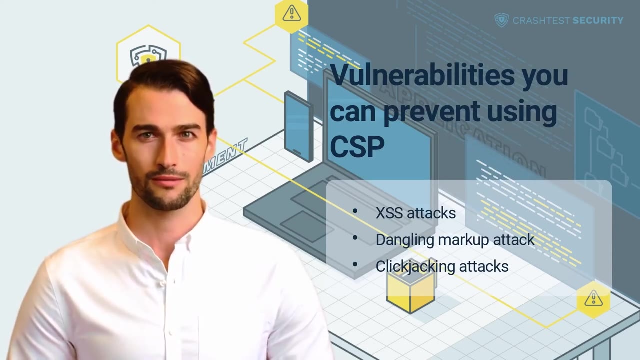 Upgrade insecure requests In websites with numerous insecure legacy URLs. this policy instructs the browser to treat every insecure URL as if it has been replaced with an HTTPS secure URL. A content security policy header Provides a framework for developers to control privilege and the loading of resources for the application process. It helps reduce the risk. 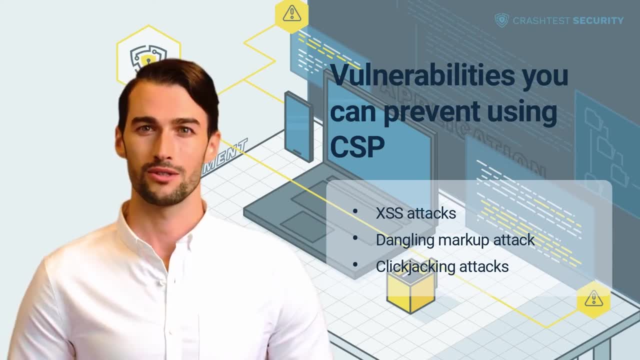 of attacks that leverage the need for loading resources within a malicious context. With properly formulated CSPs, the developers can access a reporting mechanism to detect and document security flaws exploited in production. All major browsers support CSPs, making the standard header layer of application security. 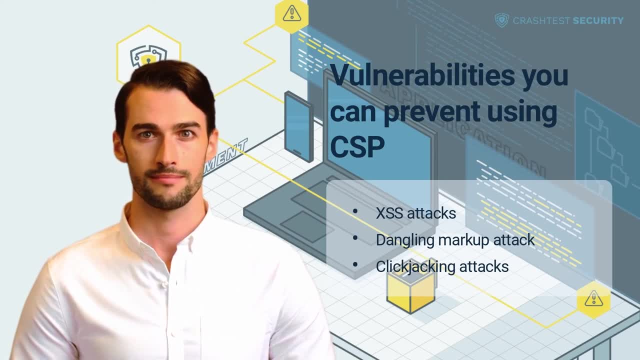 CSPS enable granular control over inline script execution, how inline styles are applied. dynamic code execution. vulnerabilities you can prevent using CSP. CSPS protect web applications from several vulnerabilities and attacks, including XSS attacks. CSPS form the first line of defense. 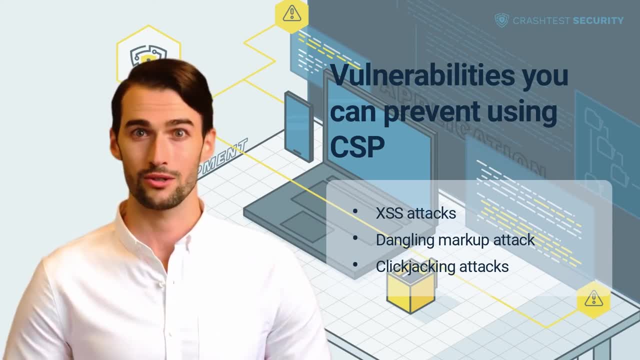 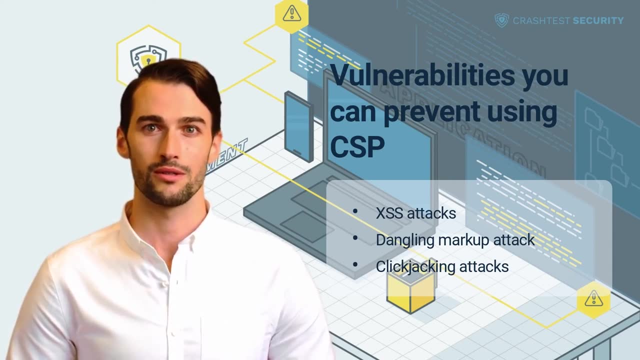 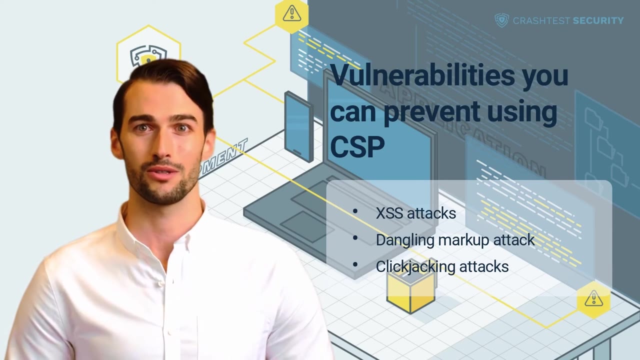 against XSS attacks as they block the execution of malicious scripts injected by untrusted sources. To reduce the XSS attack surface developers restrict loading resources using the ScriptSRC self directive. This directive only allows the page to load scripts originating from the same server hosting the page. 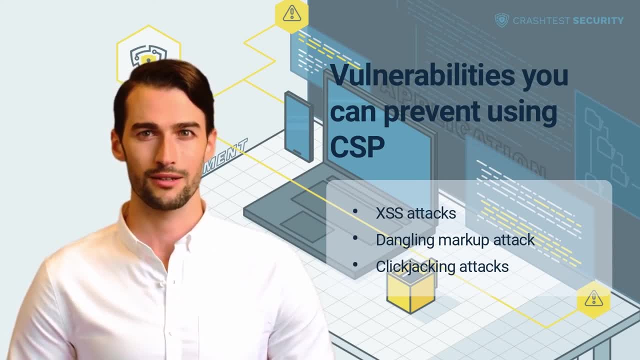 The ScriptSRC-allowed web URL enables the page to load scripts from a specific domain. Besides whitelisting resource origins, CSPS also help mitigate XSS attacks using hashes and nonces. A nonce is a random value specified in the CSP so that it is used to load scripts in a tag. 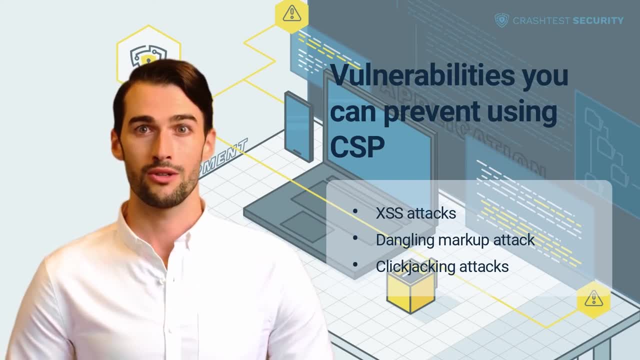 The CSP checks the nonce match source list, ensuring that the values match. Otherwise the script is executed. A hash algo component of a trusted script's contents can also be specified in a CSP directive. The script only runs when the actual script's hash. 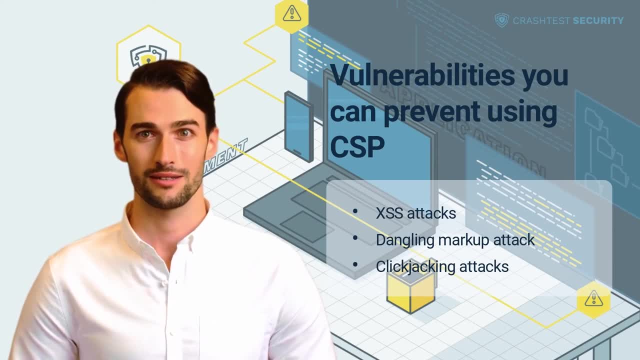 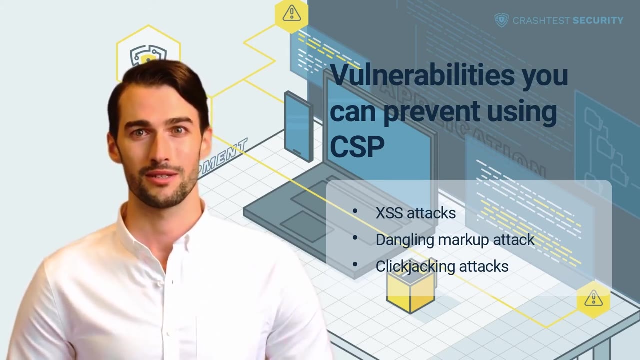 matches the value in the CSP directive. Clickjacking attacks The frame ancestors self. CSP directive governs that only pages with the exact origin can frame the policy's page. Developers can also wholly prevent framing using the frame ancestors. none directive CSPs can be used alongside 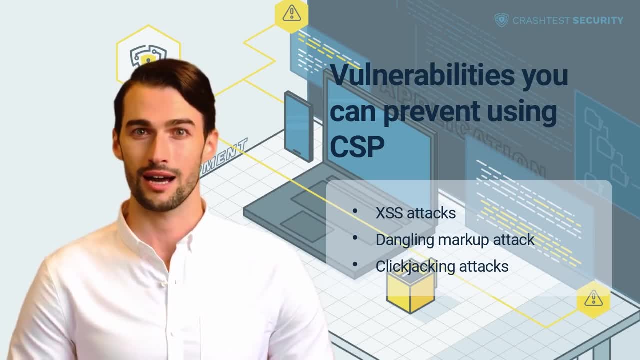 the XFrame options header to prevent clickjacking attacks. CSPs are more effective since they allow for the specification of multiple domains. The policy also validates every external resource in the parent frame hierarchy, enabling stronger protections against frame hijacking attacks, Dangling markup attacks. 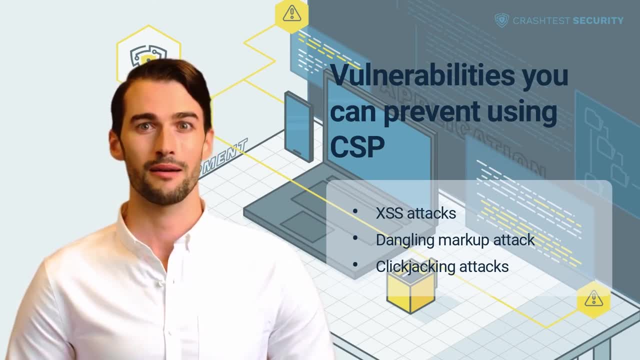 CSPs protect against dangling markup attacks by restricting the page's origin of images to be loaded. The MSRC self directive only allows images to be loaded from the exact origin. The MSRC allowed web URL directive governs the page to load images from a specific domain. 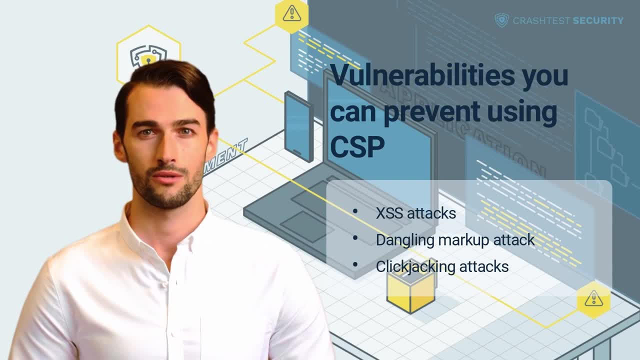 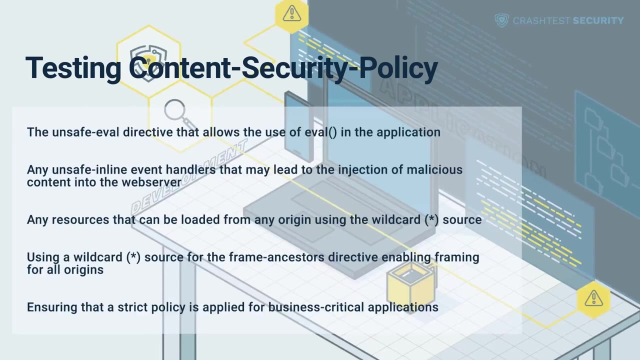 The imtag helps prevent dangling markup attacks, since it makes it easy to capture input data with minimal user interaction. Other attacks mitigated by CSPs include framing attacks, code injection attacks and cross-site request forgery. When examining the CSP meta-element content: security policy. 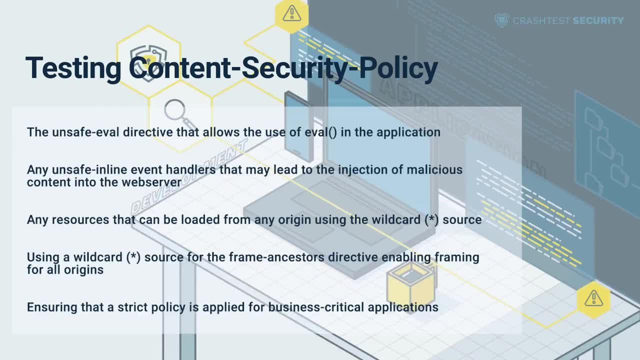 in a proxy tool. some insecure configurations to investigate include: the unsafe evil directive that allows the use of evil in the application. any unsafe inline event handlers that may lead to the injection of malicious content into the web server. any resources that can be loaded from any origin using the wildcard star source. 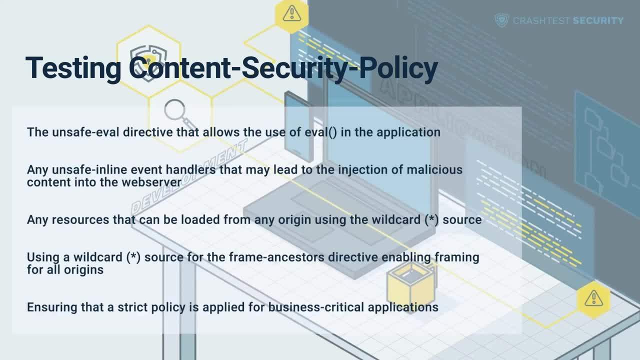 using a wildcard star source for the frame ancestors directive and framing for all origins, Ensuring that a strict policy is applied for business-critical applications. the security researcher can also use available tools such as the Crashtest Security Suite to check the strength of their security policies. 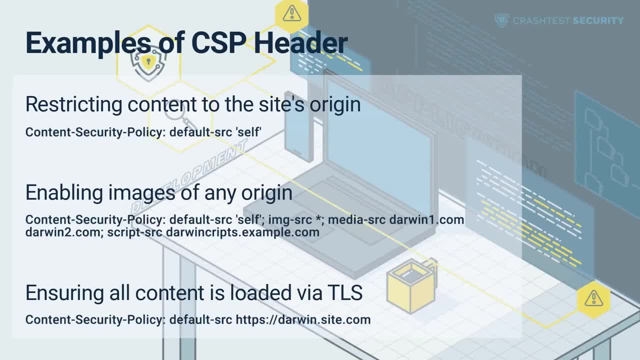 A few sample HTTP headers include: restricting content to the site's origin, enabling images of an origin and ensuring all content is loaded via TLS. Restricting content to the site's origin: To ensure all content comes from the site's origin. the web developer administrator. 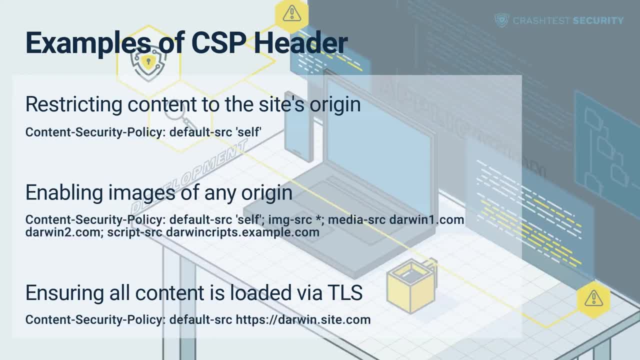 uses the default SRC directive, as shown, Enabling images from any origin. CSP allows for the specification of multiple policies for a resource by separating them using semicolons. For example, the developer can set user content to include images from any origin. restrict audio-video. 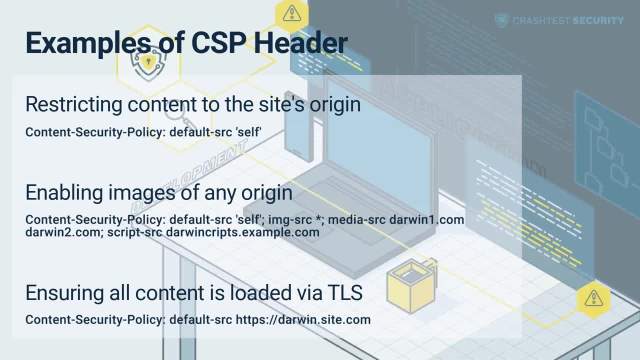 and load external scripts from a specific trusted server. as shown, Developers can prevent adversaries from eavesdropping on client requests by ensuring all of a website's content is loaded using TLS. It is achieved using the security policy shown. This policy ensures that the server only allows access. 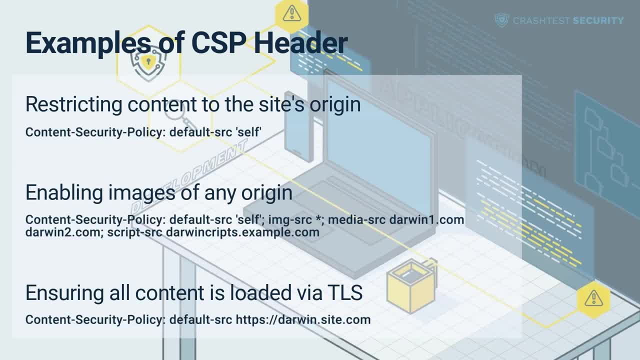 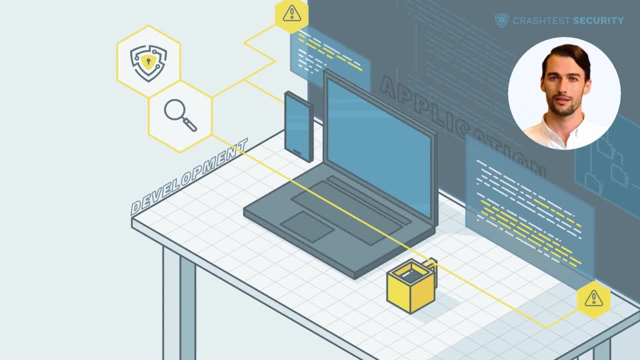 to documents loaded through the single origin HTTPS. Try Crashtest Security today to discover how it integrates into your development stack for efficient automated vulnerability scanning. The trial is free. also subscribe to the Crashtest Security channel to get more information about. 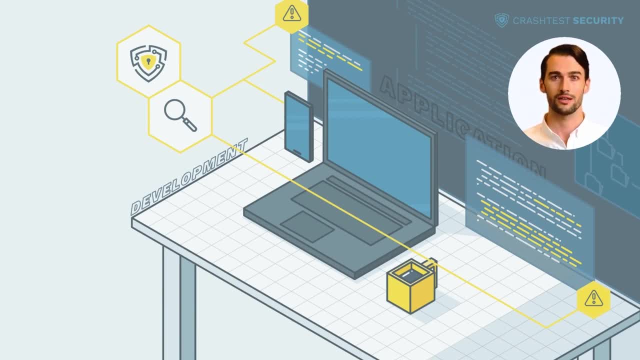 the most significant web security threats, their prevention and how to use the Crashtest Security Suite. Thank you for watching and see you in our next video.